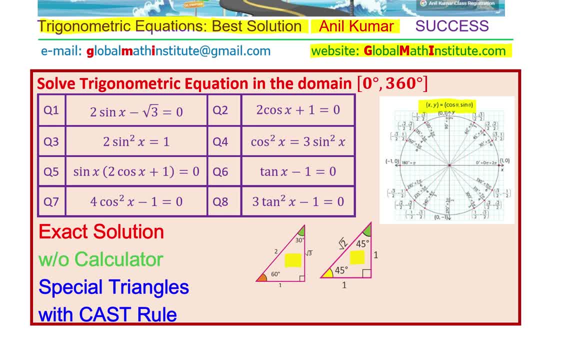 Unit circle will not be always provided to you, nor will you have a calculator. Then how will you solve trigonometric equations? The best way is to use the special triangles and the cast rule. We are going to explore and understand how to use the other rules when unit circle is not provided to you. 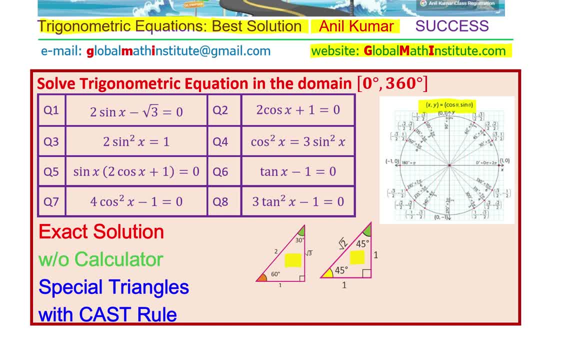 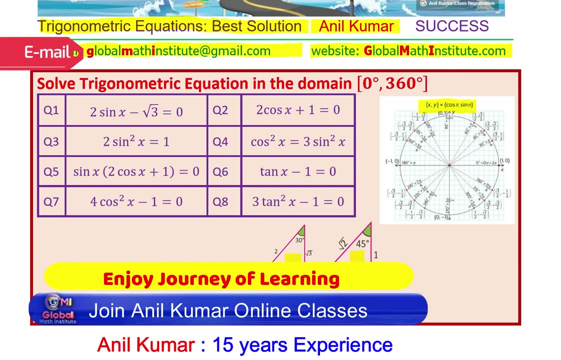 Perfect. We will find the alternate method of using the special triangles much better to find exact solution of trigonometric equations. Well, in case you want to learn from me, feel free to send an email on globalmathinstitute at gmailcom. 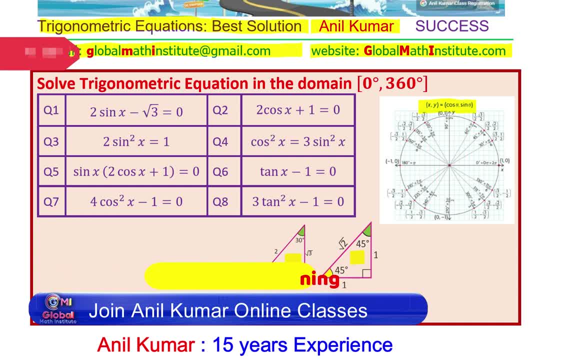 We have been serving you for last 15 years absolutely free, With more than 17,000 videos. we reach globally to more than 80 countries. You can find out more about our university. education is being provided through our channel. If you want to support, contact me on this particular email. 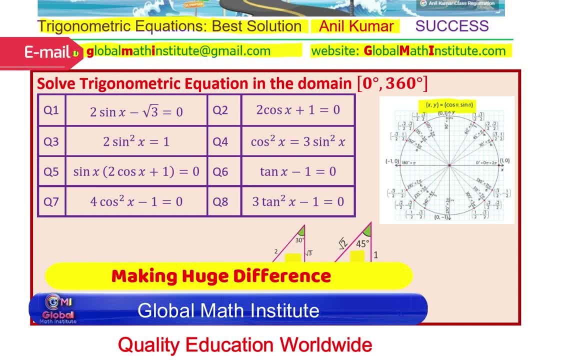 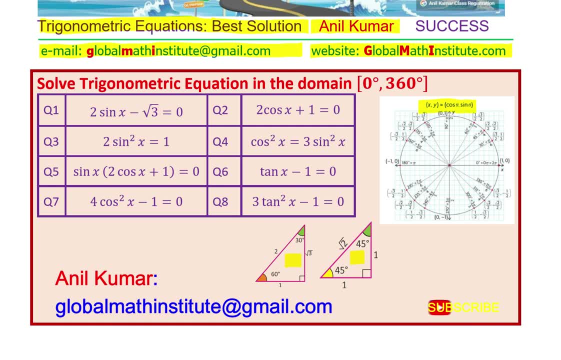 We can make a huge difference. Great, And now let's understand one by one, how do we solve these questions using both techniques: unit circle and without unit circle- Perfect. So let's talk about unit circle first. In a unit circle, any point on the coordinate on the circle will look like this: 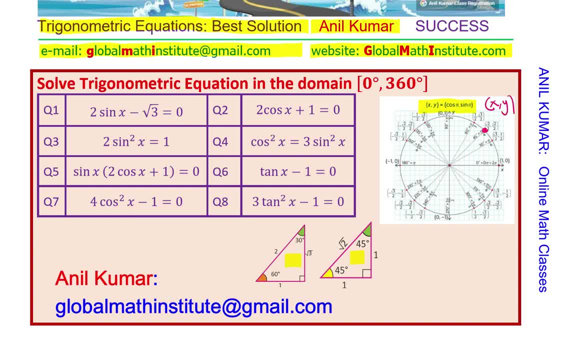 Any point on the coordinate on the circle will be given as x, y, correct. Now in unit circle the radius is one unit. So when you write the coordinate point x and y, in that case sin theta are the corresponding values. 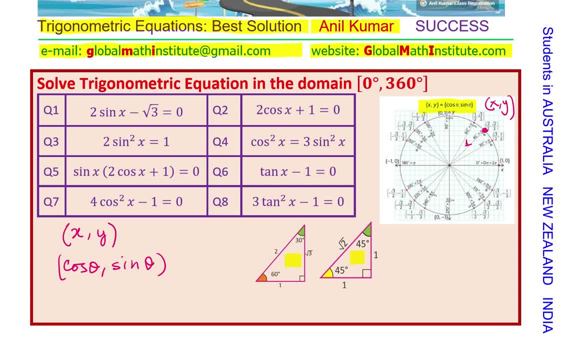 So you can read them directly from the unit circle right. So I may rewrite this as: x equals to cos theta right And y equals to sin theta. Make sense To find tan theta, of course. what will you do? Tan theta is the ratio of sin theta over cos theta, correct? 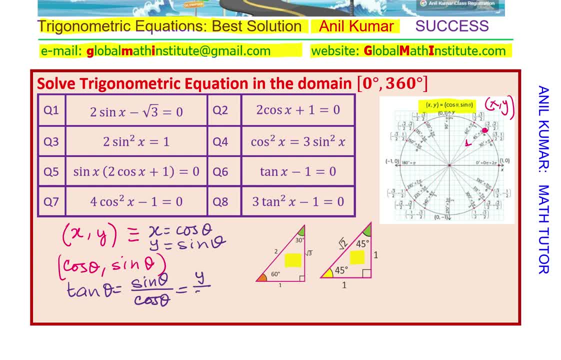 So that ratio means y over x, correct? So that is how you could read directly the values for primary trigonometric ratios from the unit circle, Then also read the values for secondary trigonometric ratios. So what we are saying here is that at any point, let's say, given here radius is one and this angle here, if it is theta, in that case x value corresponds to cos theta, y to sin theta and their quotient, the ratio y over x is tan theta. 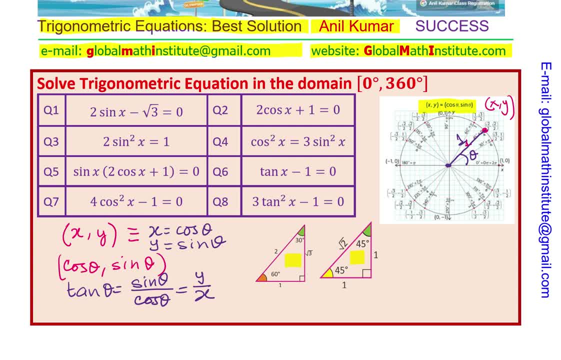 So that's one way of doing it. The other way is to use the two special triangles which I have shown. One is 60, 90, 30 triangle where the sides are 1, square root, 3, and 2, hypotenuse being 2, adjacent being 1, for 60 degrees. 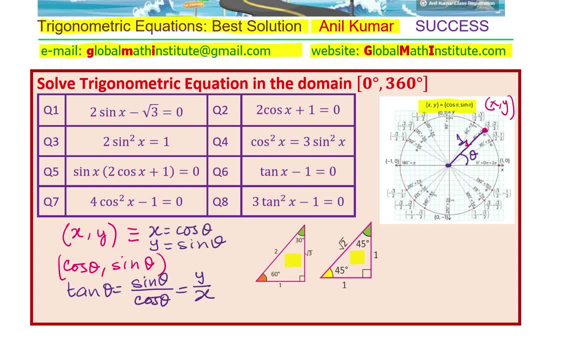 And then we have the other 45,, 45,, 90 degrees triangle where the sides are 1, 1,, square root, 2.. You could use these along with the cast rule, right? So you know in which quadrant which trigonometric ratio is positive. 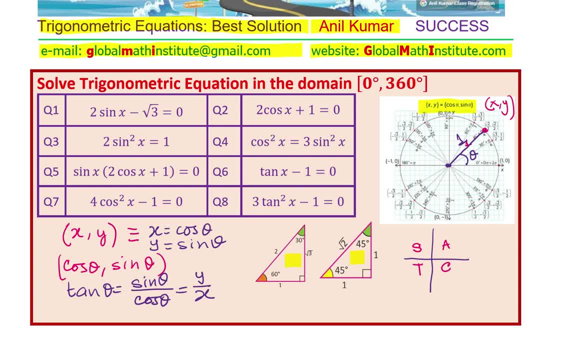 So, along with cast rule, you can apply the knowledge of special triangles to find the solution. So we are going to explore both the methods with each and every equation. So I hope it makes sense. So now let's get to the very first question. 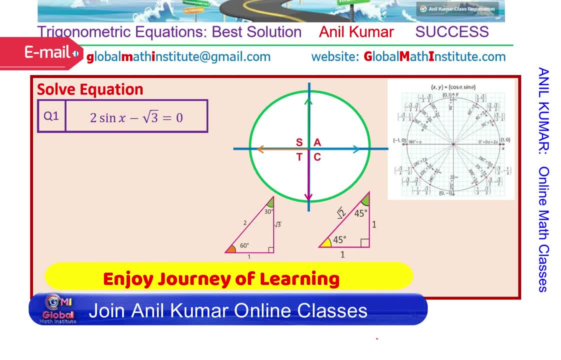 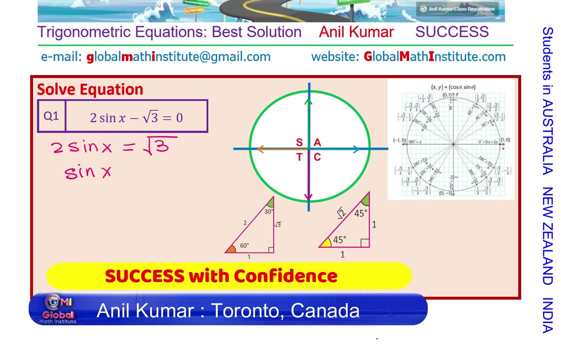 You see, what we have here is an equation which is 2 sin x minus square root 3 equals to 0.. Let's rewrite this equation as: 2 sin x equals to square root 3.. That means sin x equals to square root 3 divided by 2.. 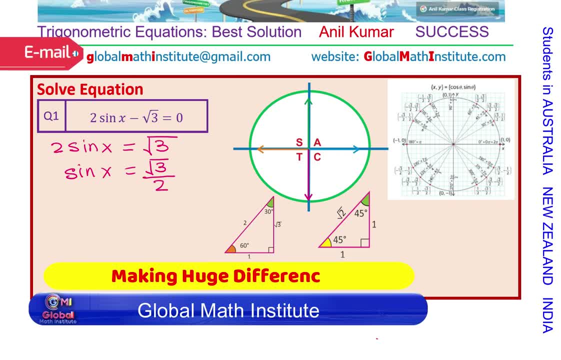 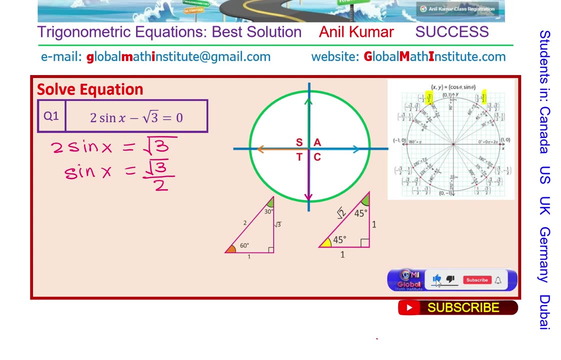 Now square root 3 divided by 2 on the unit circle. where do you get? Well, it is a positive value. So where we get here is those are the two values, correct? So you can read the two highlighted points on the unit circle. 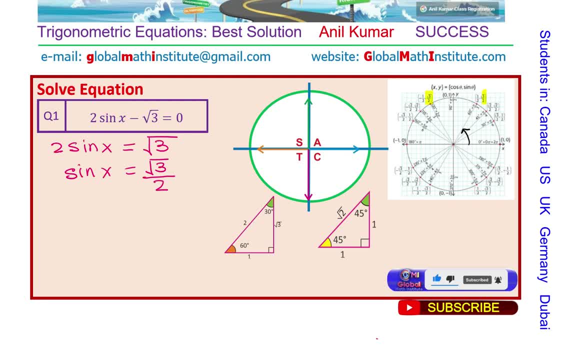 And the angle marked here, also given or written on the unit circle as 60 degrees, and it is 120 degrees, You get the idea. So we can see from the unit circle directly that we have x equals to 60 degrees and 120 degrees, correct? 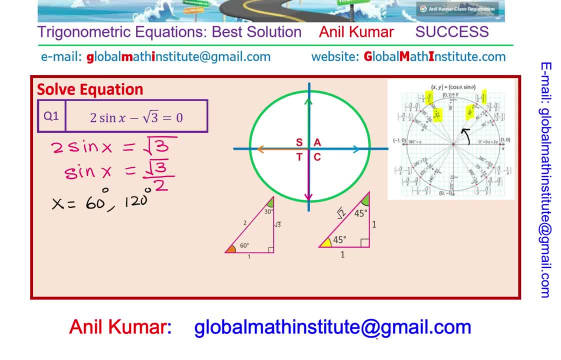 So you got the answer directly from the unit circle, But then the unit circle should be there with you And the y values of square root, 3 by 2, corresponding to the angle theta, which happens to be 60 and 120, will become your answer. 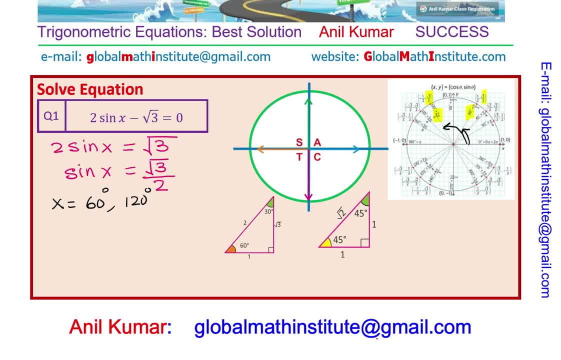 Now here is an alternate approach. So now let's look into the alternate approach. We know here that sin x is greater than 0. It is positive, right. So we know that sin x is positive, correct. So it means which two quadrants? 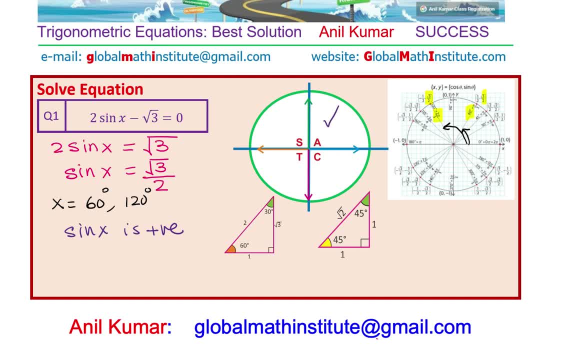 Well, we are talking about all are positive in quadrant 1 and sin is positive in quadrant 2.. And therefore we are looking for the angle in quadrant 1 and quadrant 2,, both the quadrants correct Now, since it is square root 3 by 2,. 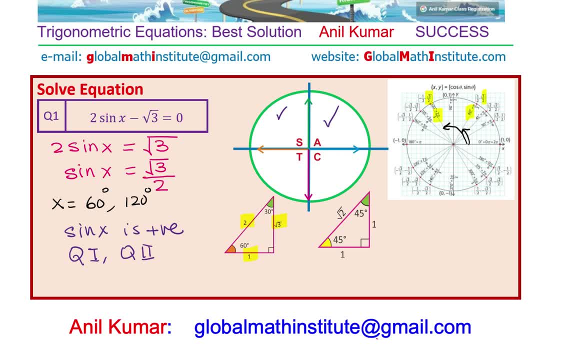 I am going to use the special triangle 30-60-90.. That is the triangle which has square root 3 as well as 2 in it. Now the ratio is square root 3 by 2 means the opposite side should be square root 3. 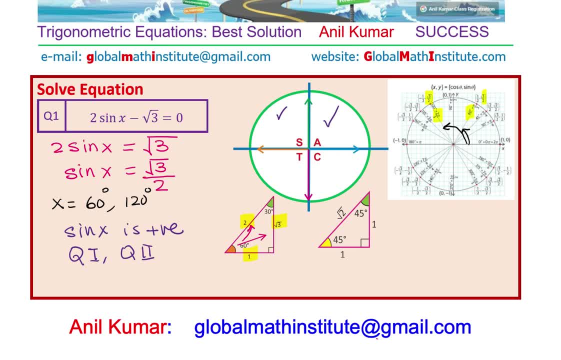 and the hypotenuse will be 2.. So that corresponds to angle 60. So we get our related acute angle 60 right there. You see that Now the other angle we know is also 60 acute. correct Principal angle will be what? 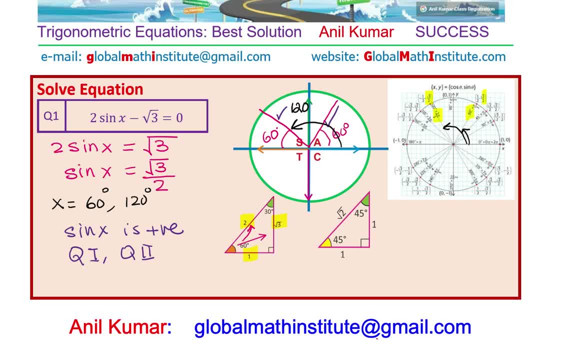 180 minus 60, and that is what you get as 120 degrees. So you get your answer exactly same, which is: x is 60 degrees and 120 degrees Make sense, But it follows a logic. Sin x is positive in quadrant 1 and in quadrant 2. 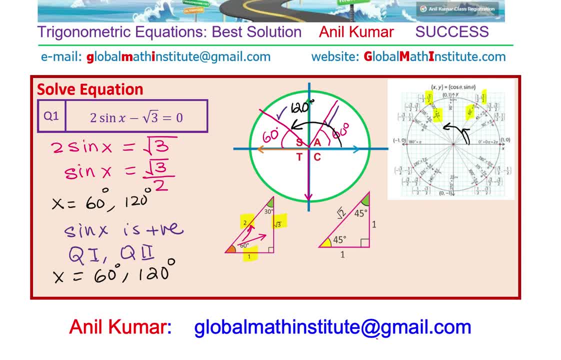 and therefore we have to look for two solutions. Since the values are square root 3 by 2, we have to look into this special triangle which is 30-60-90.. And then, which side is opposite to square root 3?? 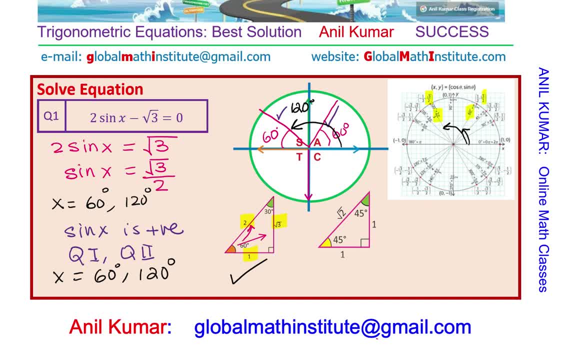 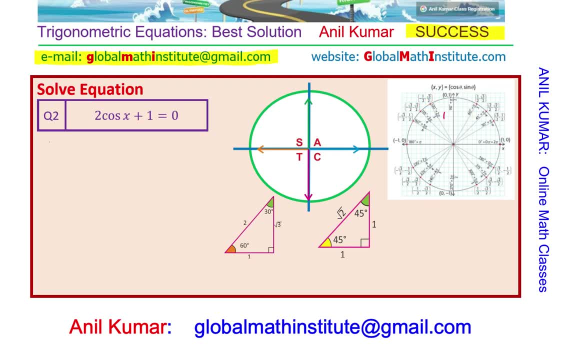 Well, the angle opposite to square root 3 is 60, and that is our answer. You get the idea right. Now we will follow the same method to do question number 2.. The question, which is 2 cos x plus 1, equals to 0.. 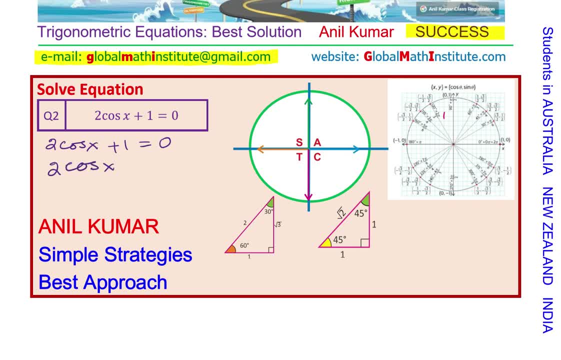 So let us isolate cos x right, Taking 1 to the other side, then dividing by 2. We get minus 1 over 2.. As soon as you get cos x as minus half, what should you think about? Well, first thing comes to our mind is about: 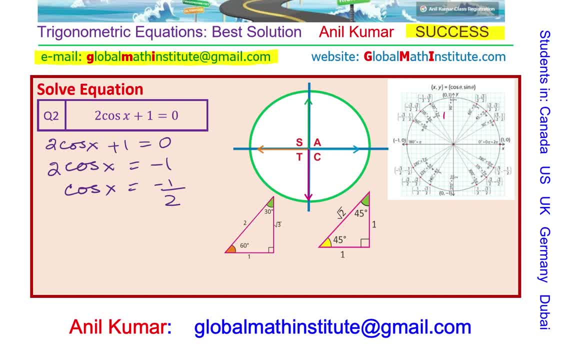 the cast rule which quadrant we have to look for. Since cosine is negative, we have to look for these two quadrants, which is quadrant 2 and quadrant 3.. You get the idea. So we know that we have got two answers. 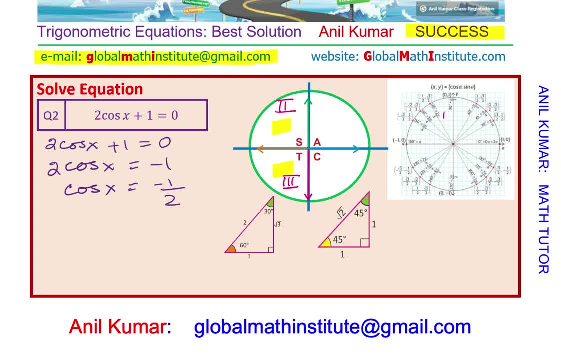 one in quadrant 2 and quadrant 3.. So you looked at cast rule before even looking at the unit circle. And then you will go to unit circle and you want the x value to be minus half. So minus half, we get 2 here, right? 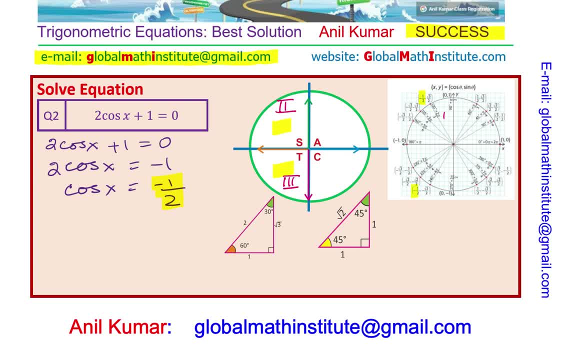 So two values, which is right there, correct, So you get two of your answers right. So there you go. Yeah, correct, So we have our answers. So if you read this, you will see this angle is 120 degrees. 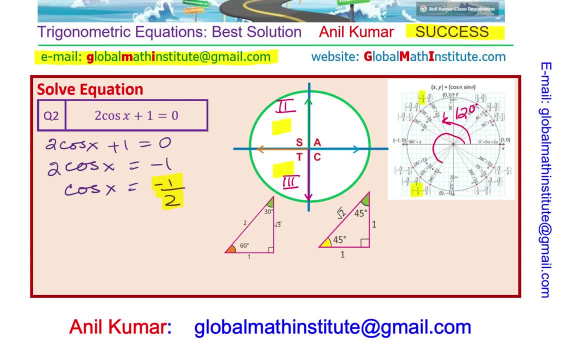 So that will be one solution. The other will be 180 plus 60, which is 240 degrees, correct? So the other answer will be 240.. And therefore you will write: x equals to 120 degrees and 240 degrees. 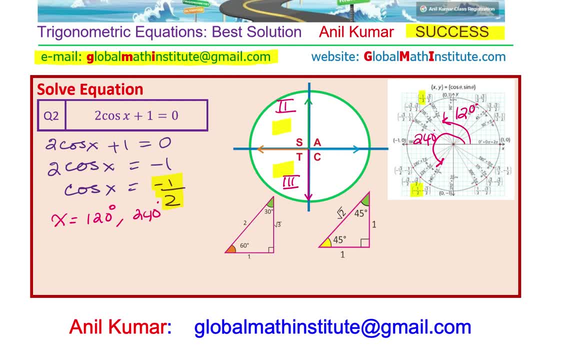 Makes sense, correct. Now, if the unit circle is like this: if the unit circle is not given to you, you may use the special triangles. I prefer to use special triangles. What do you see? You want the ratio of 1 over 2. 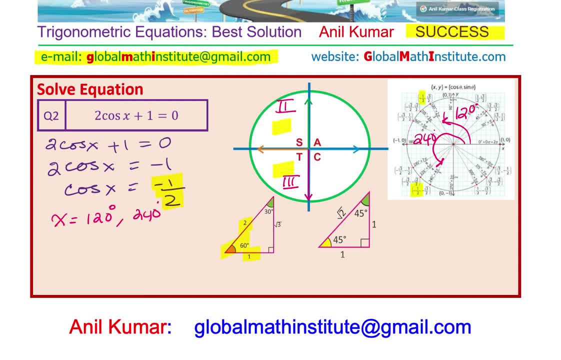 and that happens to be with an angle of 60 degrees. That means the related acute angle is 60, right, So we have related acute angle of 60. But we need solution in quadrant 2.. And in quadrant 3, correct? 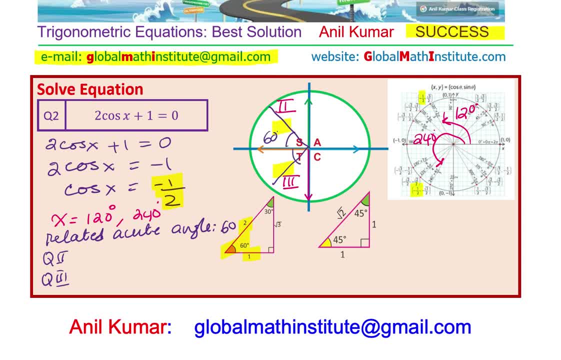 So, in quadrant 2 and 3,, if this angle is 60 degrees, what should be the answer? Well, clearly, the answer will be 180 minus 60,, right, Which is 120 degrees, And the other one will be 180 plus 60,. 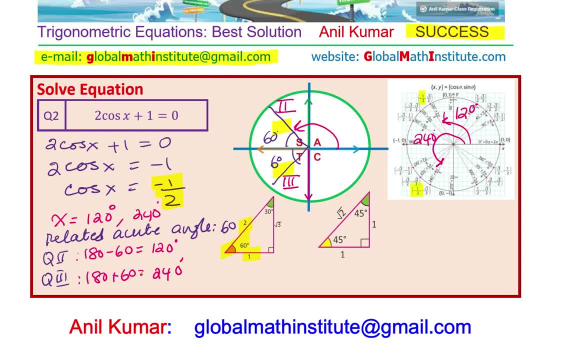 which is 240 degrees. This is a very logical step to solve any trigonometric equation. So if your basics are right and if you know the right way of doing it, you'll actually be solving trigonometric equations far more easier than with the unit circle. 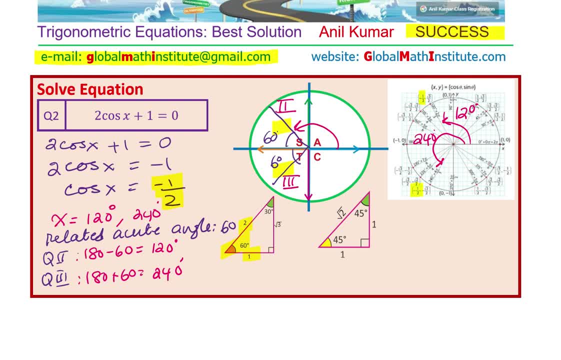 You get the whole idea right. Unit circle is only to read and match and write down the answers. It is not using brains. correct, Perfect. Now let's go to the next question, which is question number 3.. Once again, we'll follow the same strategy. 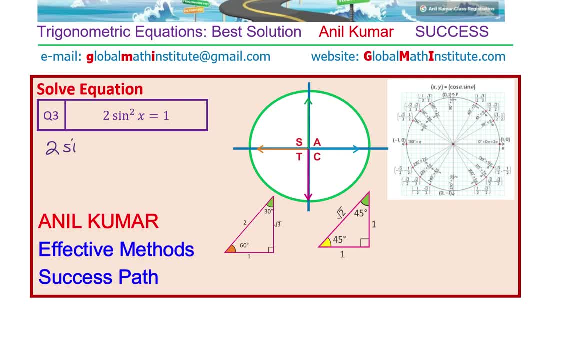 And that is we have 2. sine squared x equals to 1 isolated sine right. So sine squared x equals to half and sine x equals to plus or minus. Whenever you square root, you have to do plus and minus, which is plus and minus 1 over square root 2.. 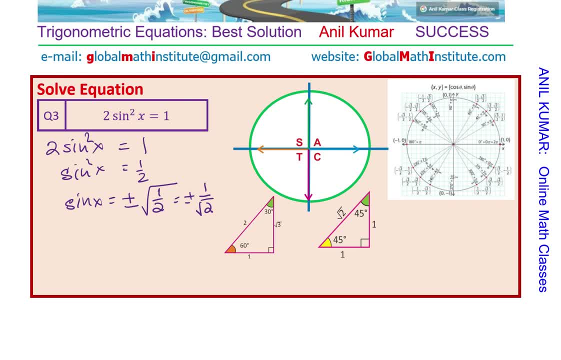 So now you know it is plus and minus means all 4 coordinates correct. So we have got 4 solutions to this. wherever the sine x value is 1 over square root 2.. So you know it is for 45 degrees acute angle. 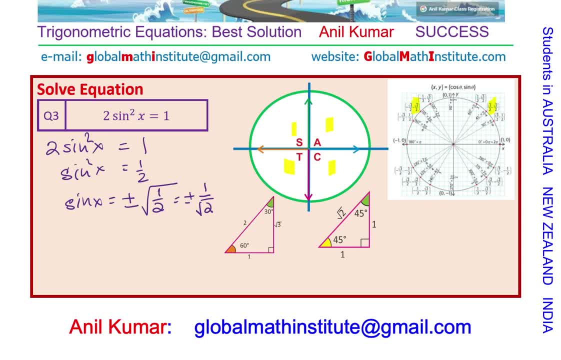 and therefore you can highlight these solutions and write down the y angle corresponding to these correct. So, from the unit circle, you can definitely read the angles and then write it down. How am I going to do it with my special triangles? Well, 1 over square root, 2 gives me an angle of 45.. 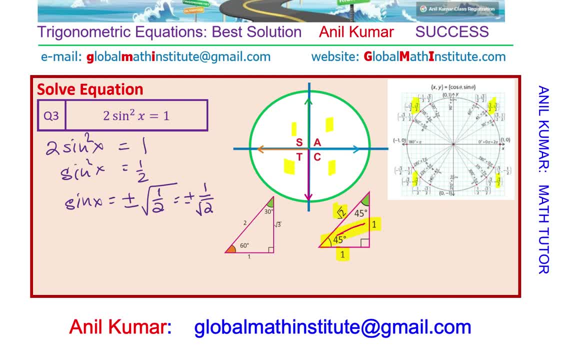 The side opposite is 45, right. So look at this side right Opposite side is 45, and it is called 1 over square root 2.. So 45 degrees is my solution in each coordinate. You get the idea correct. 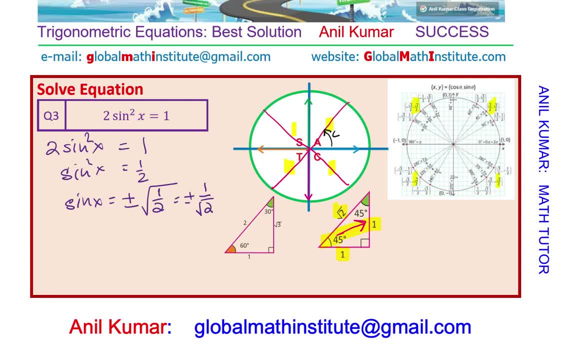 And therefore, when this is 45, first answer is 45. This is all. these are 45, correct With these are the related acute angles, but you have to always write principal angle. So principal angle will be x equals to 45 degrees, right. 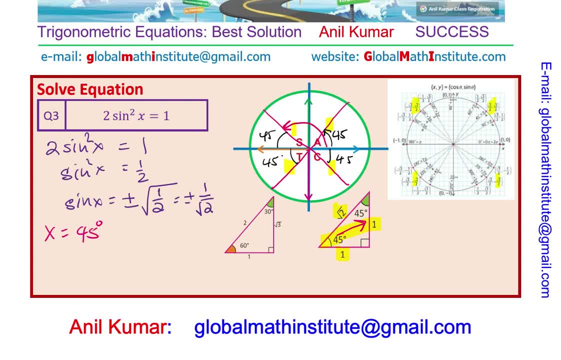 And then 180 minus 45, right, Which is 135 degrees. And then it is this angle: 180 plus 45, right, So 180 plus 45,, so 225 degrees, And then we have the last example answer. 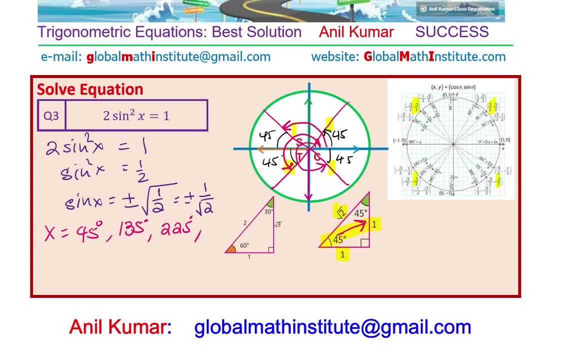 which is 360 minus 45, right, So 360 minus 45, 315 degrees, correct? So we have all the four answers which you could also read from here, correct? So you could read from this circle also and write down your answers. 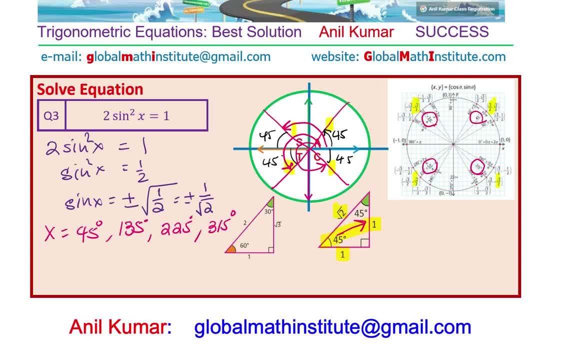 But if you are too much dependent on the circle, if it is not provided, it will be very difficult for you to write down the answers. And let me assure you it will not be provided as you move forward from your first lesson to the next lesson of trigonometry, correct? 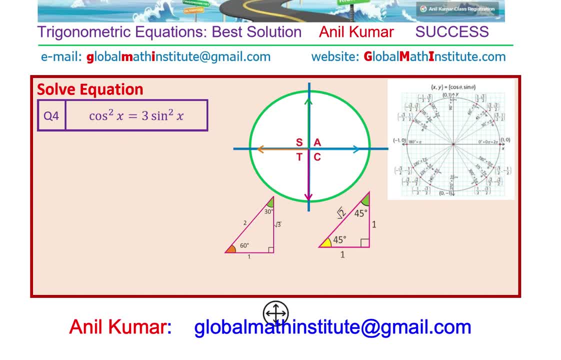 So we know now how to use our special triangles right. Even if the unit circle is given to us, I think it is better idea to use the method of checking in which quadrant the answer lies, and the special triangles. We have question 4 here. 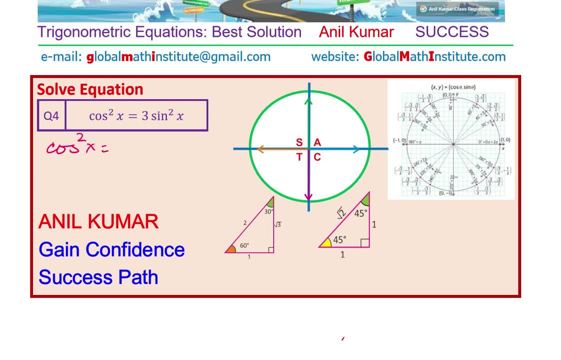 where the equation is: cos square x equals to 3, sine square x, right Isolate. but see sine and cosine ratio, you remember, is 10.. So we will divide by cos square x, we get 1 equals 2, right. 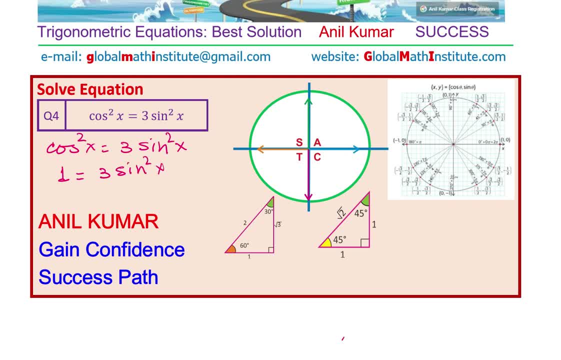 We get 1 equals 2, 3.. Sine square x over cos square x, perfect, Okay, And we can also rearrange 1 over 3. is sine square x over cos square x is tan square x correct. 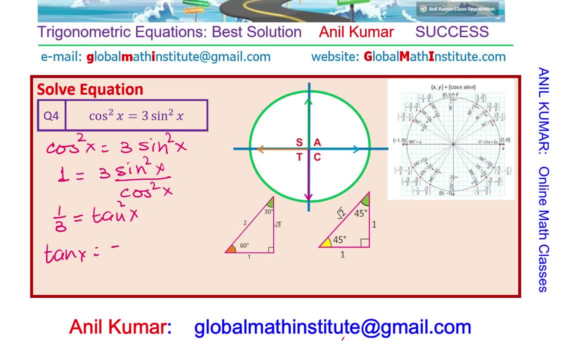 So we can write what is tan x equals to. Tan x equals to plus, minus 1 over square root 3.. Now, as soon as you get to, tan x equals to 1 over square root 3, plus and minus. So in the unit circle, 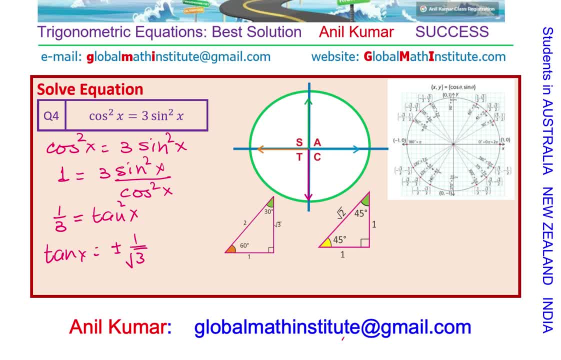 it now becomes slightly more difficult. You have to not divide the y values by x values, correct? So for this you have to see where y over x is equal to 1 over square root 3, right? Well, of course, we need solution in all the quadrants. 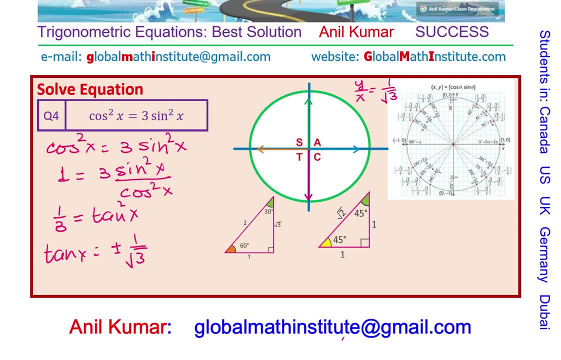 So you see how unit circle becomes difficult as soon as we move on to tan. Now let's look into our standard way. We're looking for plus and minus. That means all quadrants, right, Okay? And then, because it is involving square root, 3,. 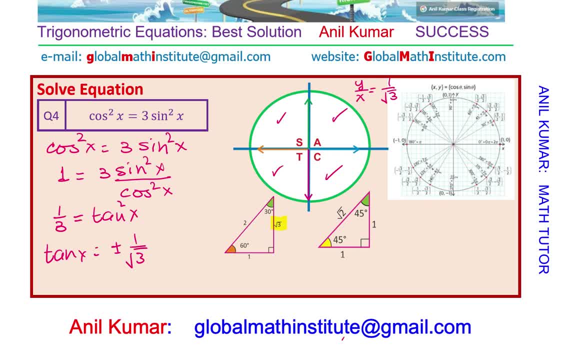 so we'll highlight square root 3 and use the triangle, which is 30,, 60, 90.. Tan is a ratio of opposite over adjacent, and therefore the angle is 60 degrees. So what do we have? We have x values as equals to 60 degrees. 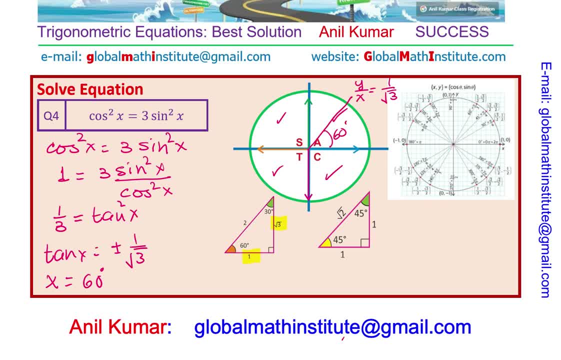 as one of our answers related acute angle- 60 degrees. So now we know, actually all the solutions will be based on acute angle of 60. So the other angle is this one, which is 180 minus 60, which is 120 degrees. 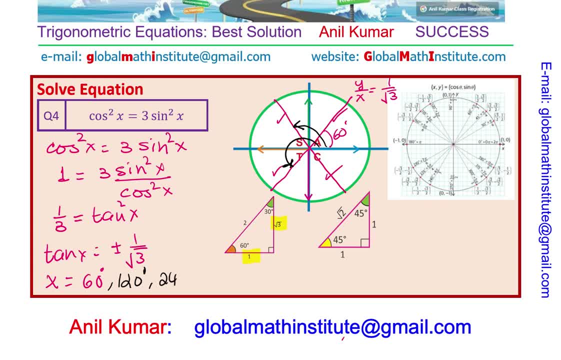 Then we have 180 plus 60, which is 240 degrees, right. And then we have 360 minus 60. So we have 300 degrees. You get the idea. It becomes extremely simple when we use special triangles and the cast rule. 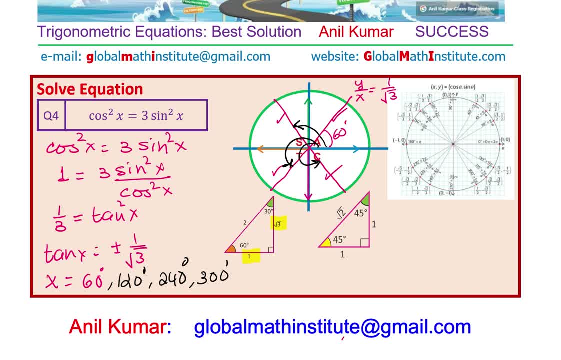 to solve trigonometric equations. I hope it is making sense. Well, in case you want to learn more, you can always contact me on globalmathinstitute at gmailcom. Now we are almost at the end. Here are the last two questions. 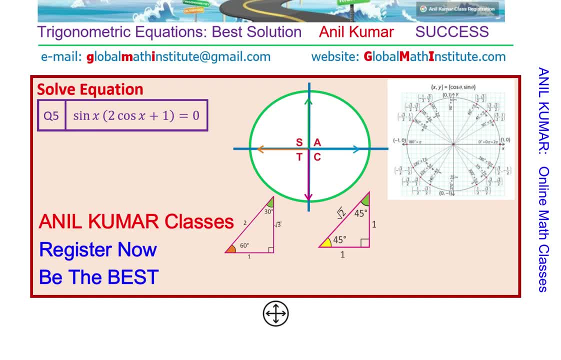 I'd like you to pause the video, answer them. Use the method of your preference. You may use the unit circle, You may use special triangles, with the cast rule right. So let's do it. We have sine x times 2. cos x plus 1 equals to 0. 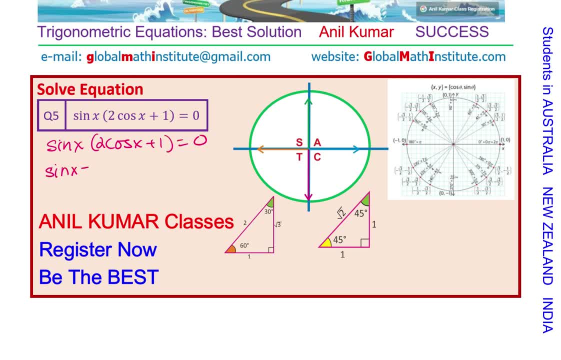 It really means we are solving two equations. One is sine x equals to 0. The other one is 2 cos x plus 1 equals to 0, means cos x equals to minus half, correct? So let's find solutions When sine x is 0,. 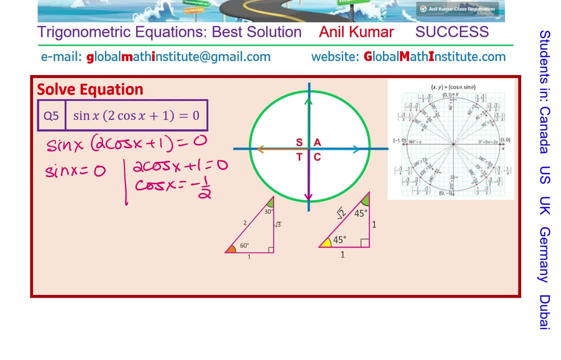 means the y value should be 0. So y value in this case is 0 at 0, right and at 180 degrees. So we get x equals to 0 degrees And 180 degrees, correct, So also 360 degrees once you complete it. 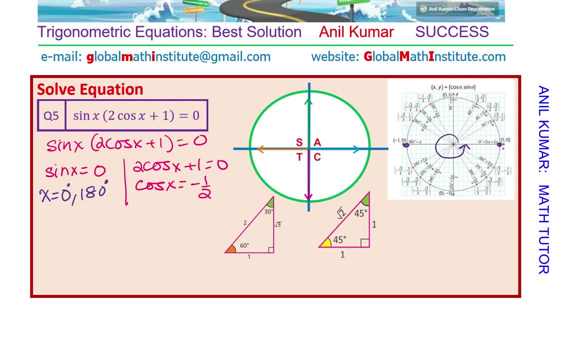 full circle, then again 360 degrees, So we'll write 360 degrees also, Since we are looking into the domain from 0 to 360 degrees. for all our answers clear Now: when is cos x equals to minus half? So, as we said, if I use the triangle, 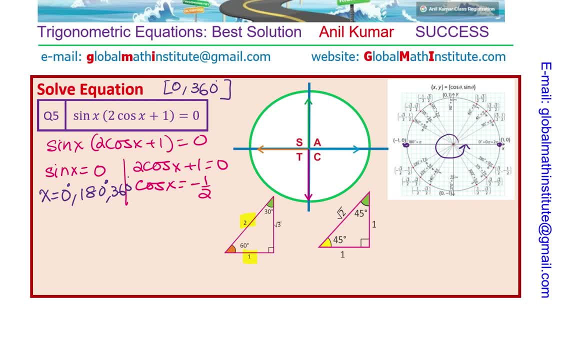 which is special triangle ratio of 1 over 2 is what we are looking into, The acute angle being 60, right, So now let us see the solution, for cos x equals to minus half. Well, cos x equals to minus half means. 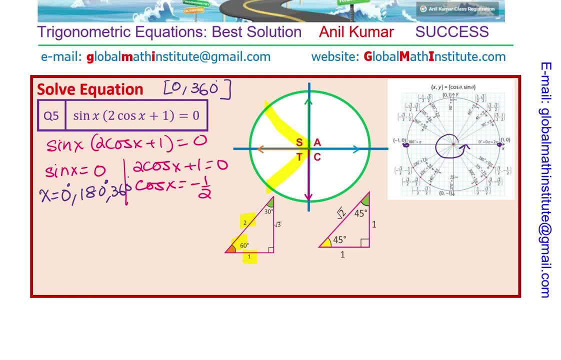 we are in quadrant 2 and 3, related acute angle being 60, correct? So if that is the case, the two answers will be these: right: 180 minus 60,, which is 120 degrees, and 180 plus 60,, which is 240 degrees. 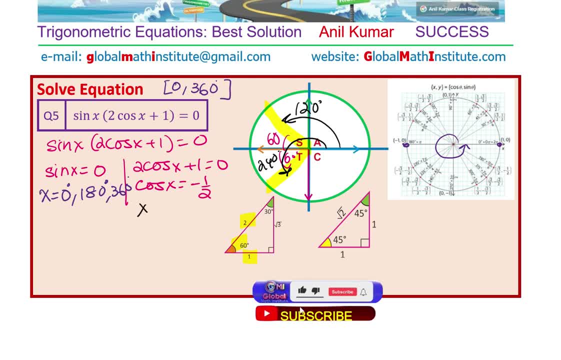 Make sense. So we can write down this: x equals to 120 degrees and 240 degrees. Is that clear to you? So there are five answers for this particular equation, which we just did, So I hope it's making sense right. 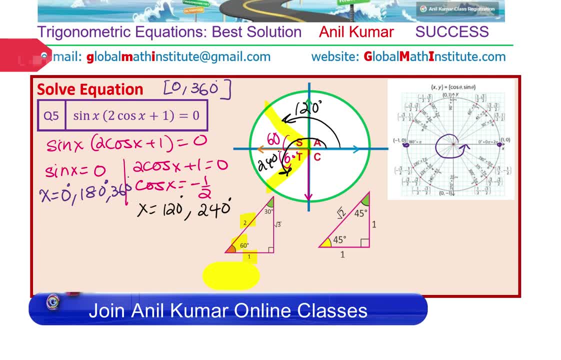 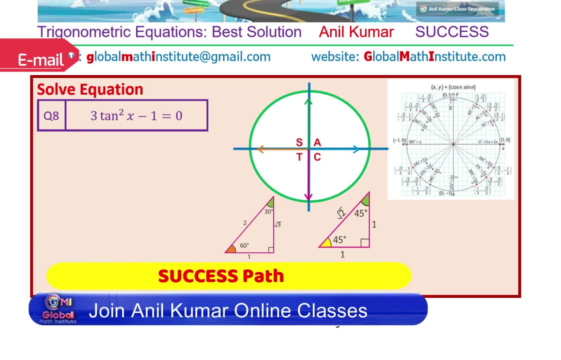 Okay, great, Now let's move on and take up another question, right, So I'll take up another question on this. So this is going to be our last question to solve. We can use any method. You can use a unit circle. 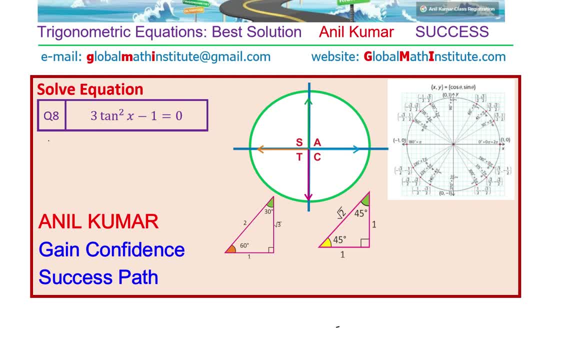 special triangles, along with cost rule, whatever you need. Let's write down the equation, which is 3.. tan square x minus 1 equals to 0 means tan square x equals to 1, and 1 over 3, and tan x will be equal to plus or minus. 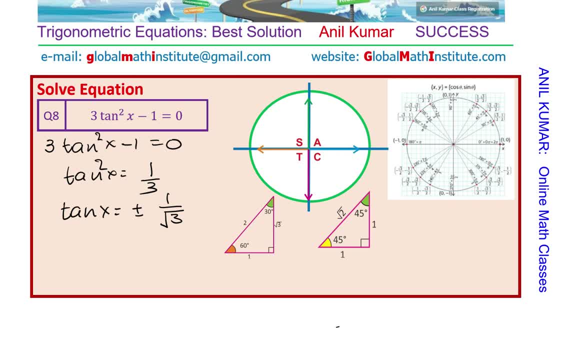 1 over square root 3, correct. So when you get 1 over square root 3, square root 3 is involved. that means the special triangle will be 30,, 60, 90.. 1 over means this.